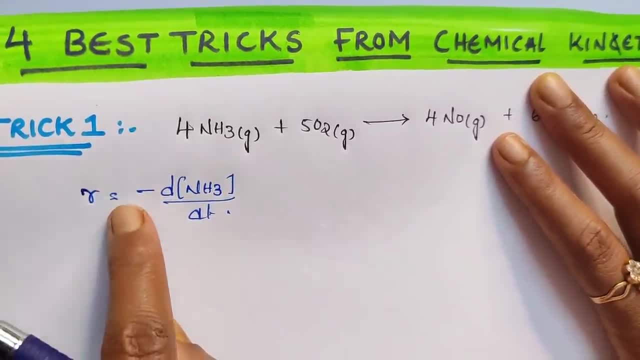 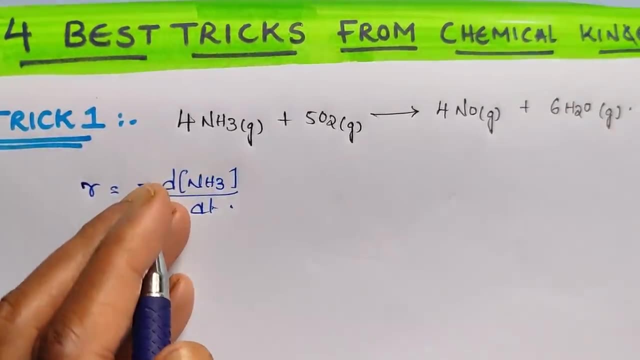 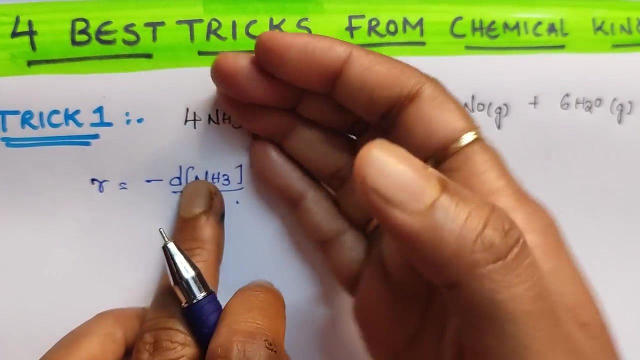 need to do is first you have to write the rate expression Rate equal to you know. reactant concentrations decreases with respect to the time When reaction proceeds. its concentration decreases. What do we need When it decreases? this term becomes a negative. 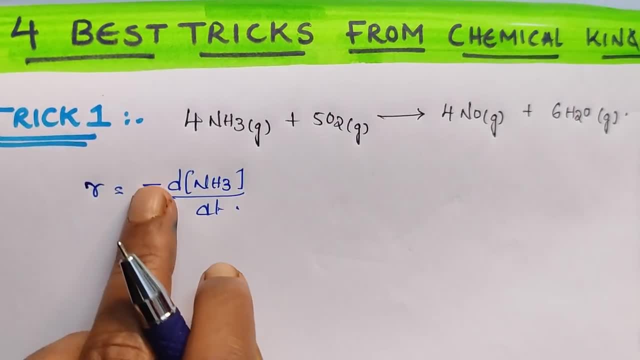 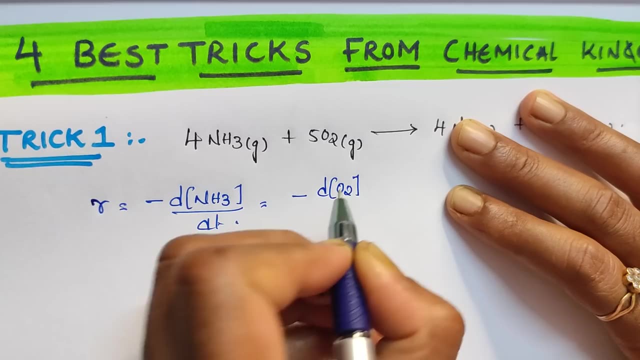 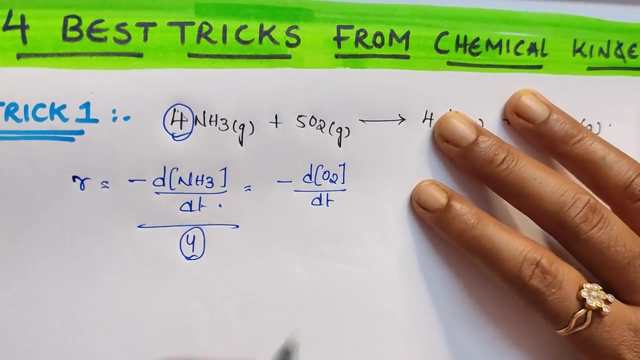 A rate can never be negative. To make it a positive, we keep some negative term before that. Here you know. I want to tell you only this expression formula: Whatever the stoichiometric coefficient is there, just write down that Here stoichiometric coefficient is 5.. So 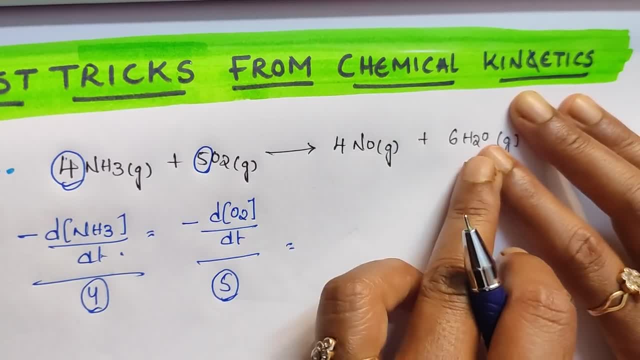 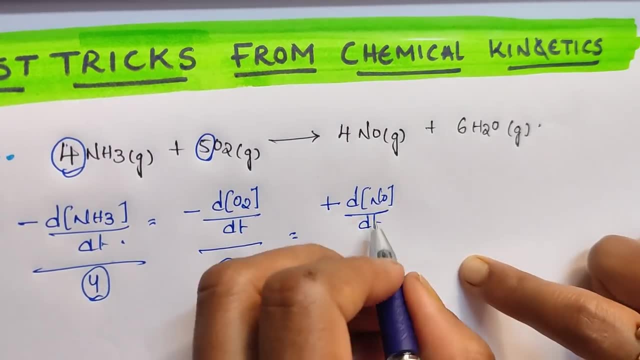 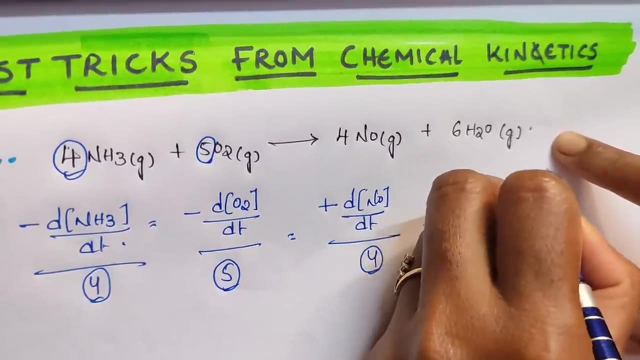 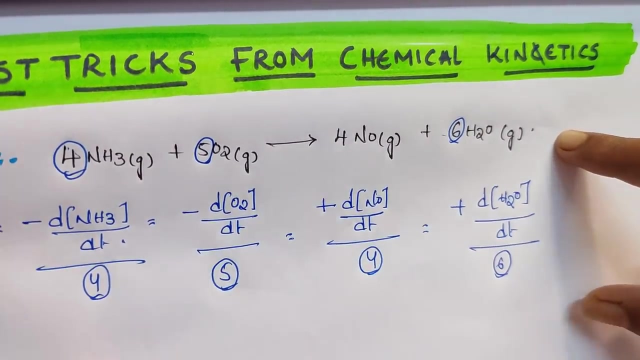 write 5 over here And product concentration always increases. So plus D of NO concentration with respect to the time divided by stoichiometric coefficient is 4,, which is equal to plus D of H2O divided by DT. Here stoichiometric coefficient is 6.. Once you write the rate, 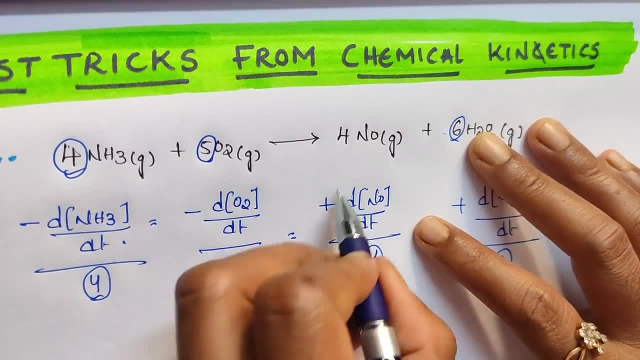 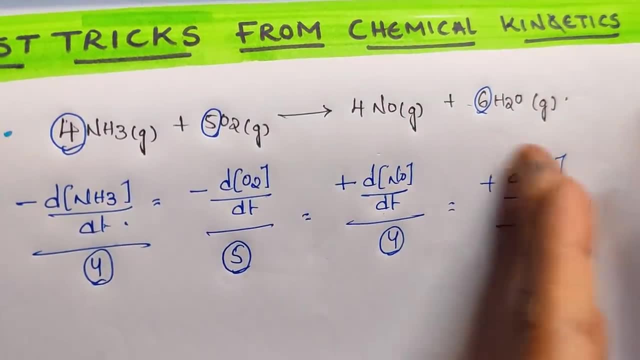 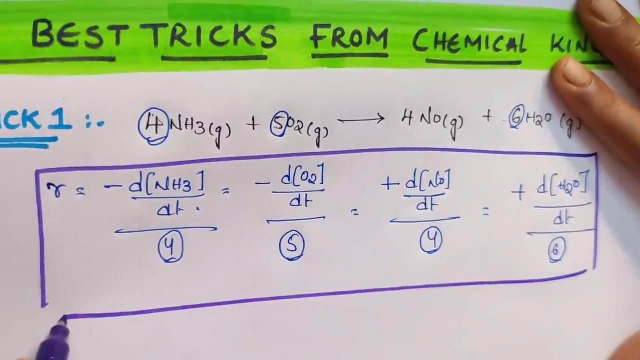 like this: Whatever they have given in a question, if they have given D of NO by DT, substitute it, Substitute that value in this place and relate it. If you write first, you know expression like this, you do not get any confusion. Now let us see one question. This is the. 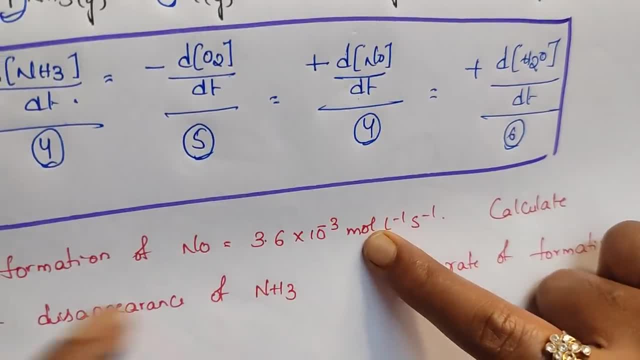 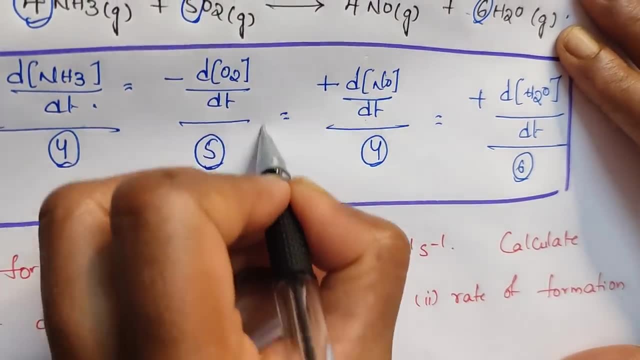 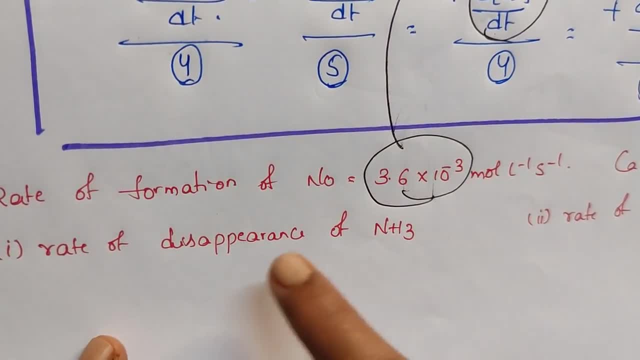 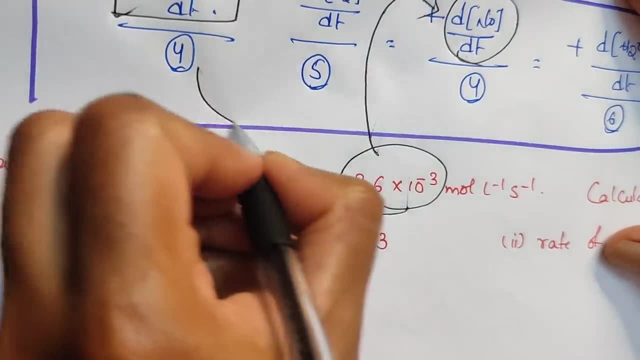 rate expression of this. And they are asking calculate rate of disappearance of ammonia. So they are asking this expression, This they are asking. So just relate these two and write the expression minus D of whatever they asked in a question. They asked rate. 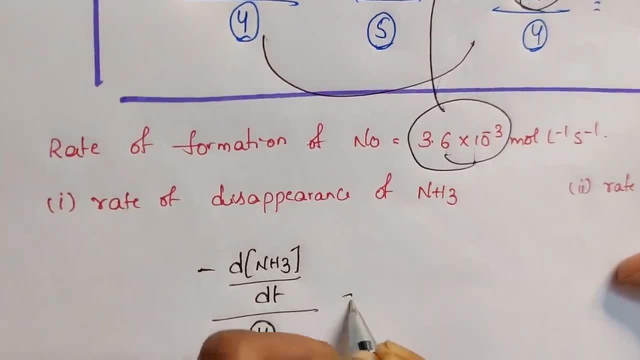 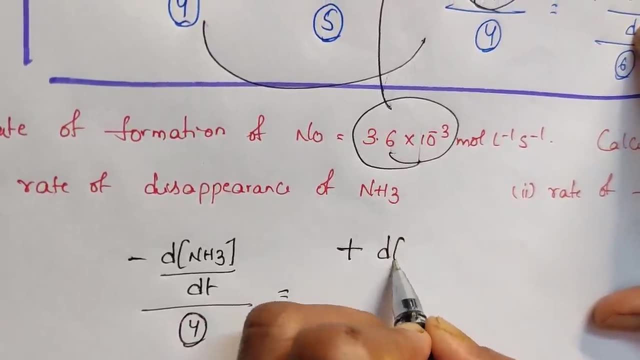 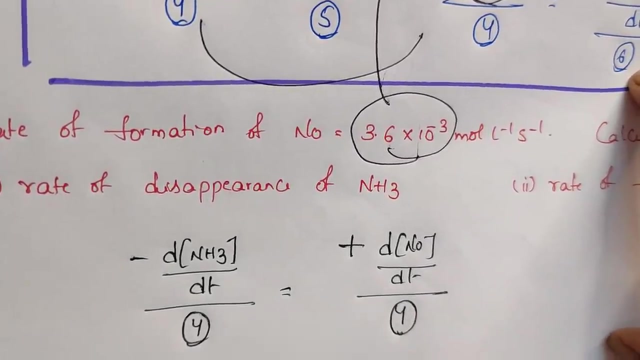 of disappearance of ammonia. Okay, this is the expression. Whatever they are, in a stoichiometric coefficient, divide it and you know. plus, with respect to what NO is given instead of NO, if H2O is given, then take H2O expression. whatever given in a question, take that expression. 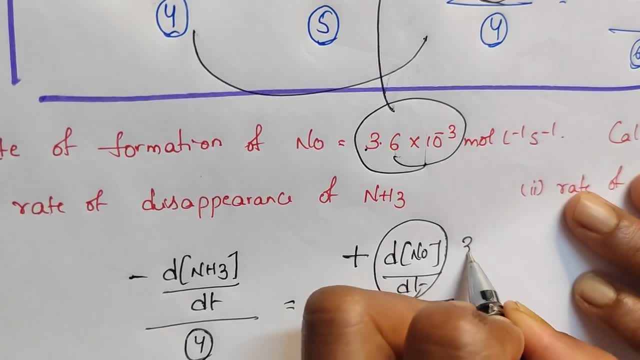 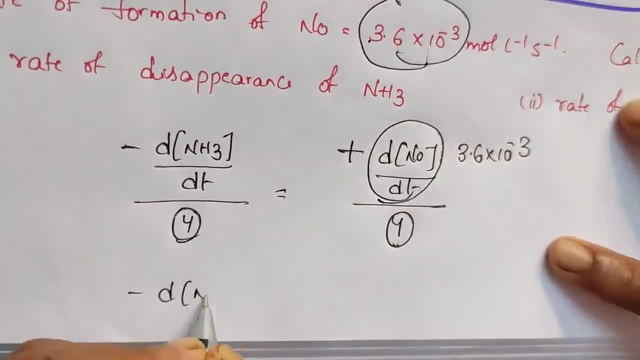 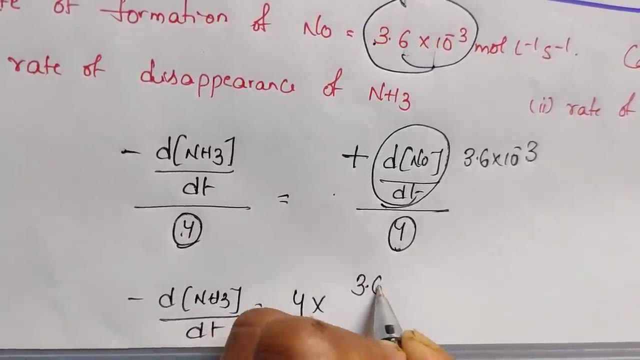 and here the value is. this value is 3.6 into 10 power of minus 3. substitute directly after that minus D of NH3 by DT, which is equal to move this 4 this side, then 4 into 3.6 into 10 power of minus. 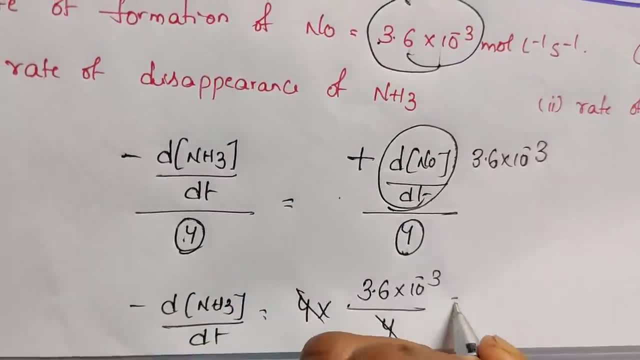 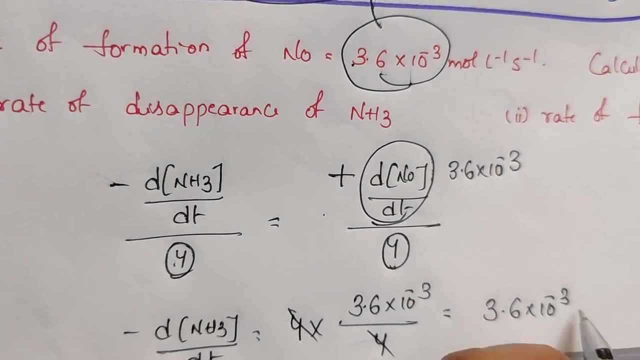 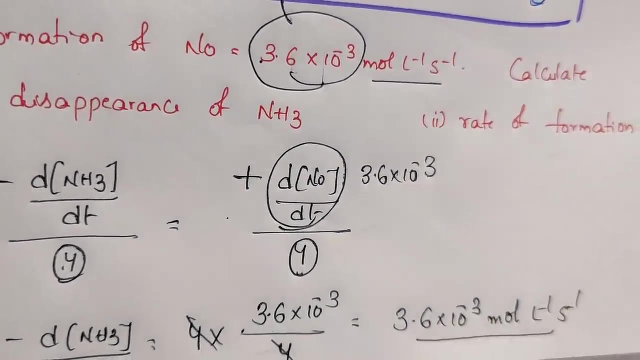 3, its value given in question divided by 4. so ammonia formation also same as that of you know ammonia disappearance is equal to rate of same value we are getting unit is, whatever unit is given here, easy, it's very easy, directly substitute that now rate of formation. 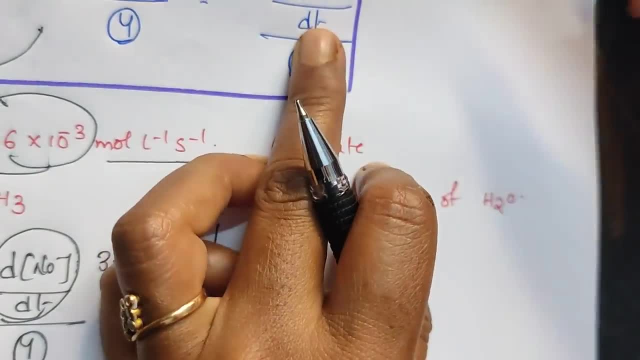 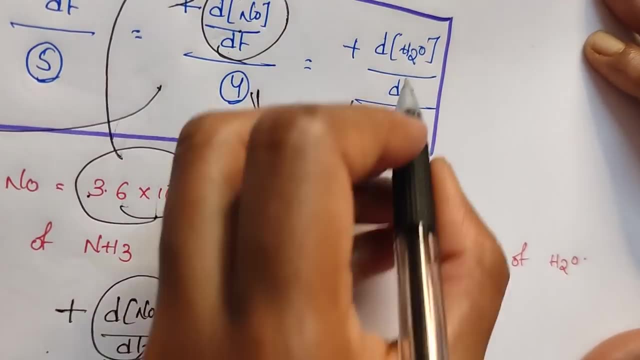 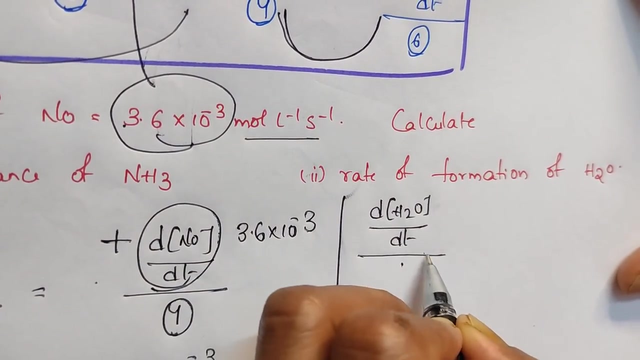 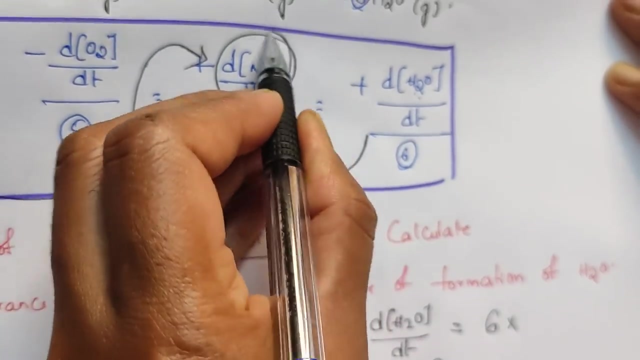 of H2O. how to do that? they're asking rate of formation of H2O and they have given this data, so you need to take these two expressions. then we want: D of H2O by DT divided by stoichiometric coefficient is 6, then I move this 6 toward this side, then multiplication 6 into its value already. 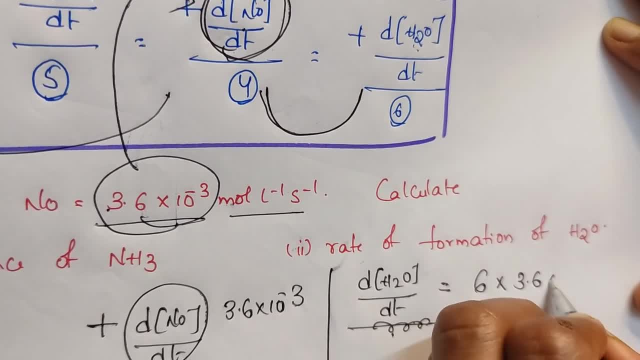 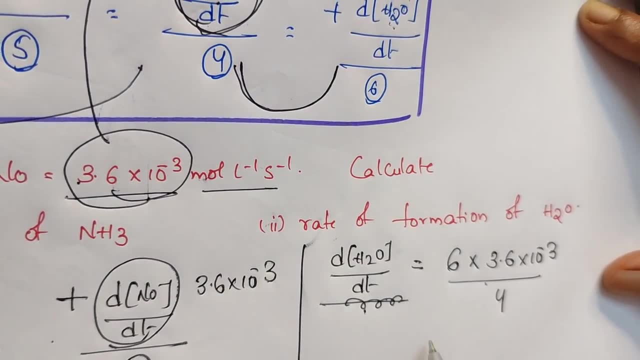 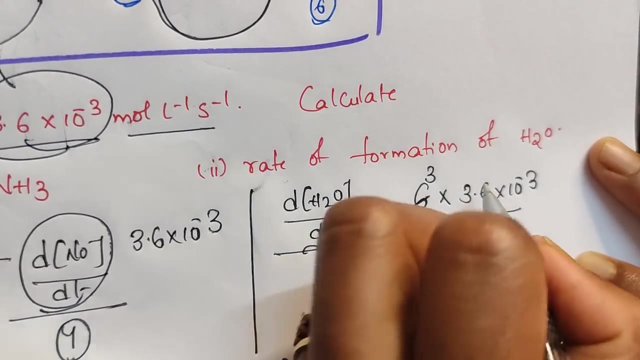 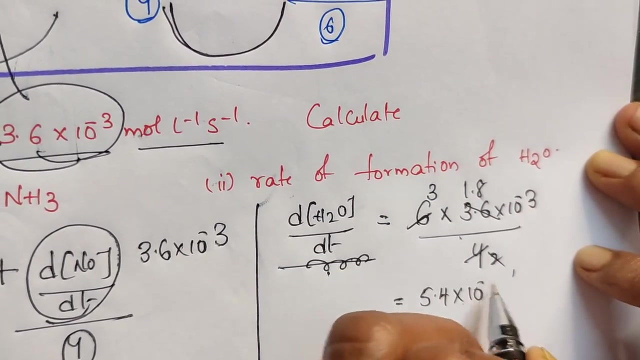 given in a question: how much 3.6 into 10 power of minus 3, divided by what is the stoichiometric coefficient of this 4? then solve this one. you will be getting to 2 sir to 3 sir to 1 sir to 1.8 sir. so 3 into 1.8, 5.4 into 10 power of minus. 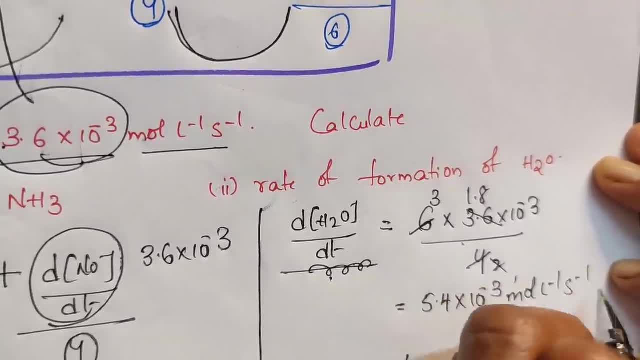 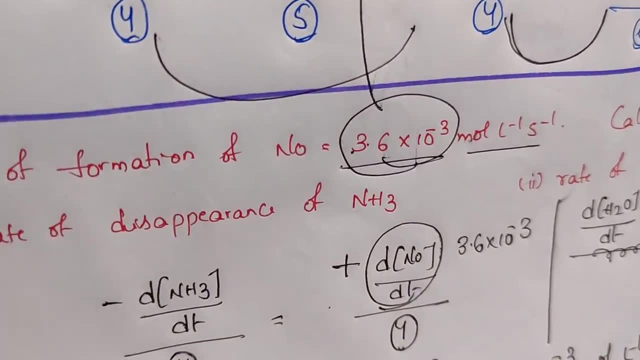 3 unit is already given in a same unit. you just write over here and select that option. this is the way to solve. I'll give you the test yourself question based on this tricks at the end of this video, so that you can try it out then. 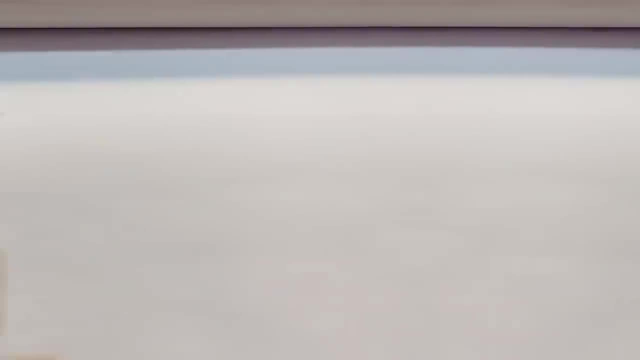 you will come to know. now let's see the trick number two. they ask you relation based questions like T 99 percentage is equal to how much of T half or T half? they will give you in a question. they ask you T 99.9 percentage. for a first. 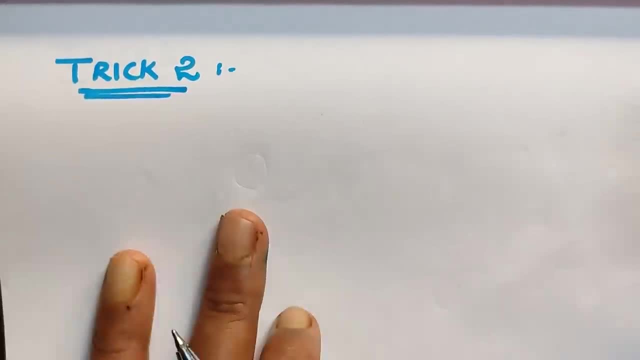 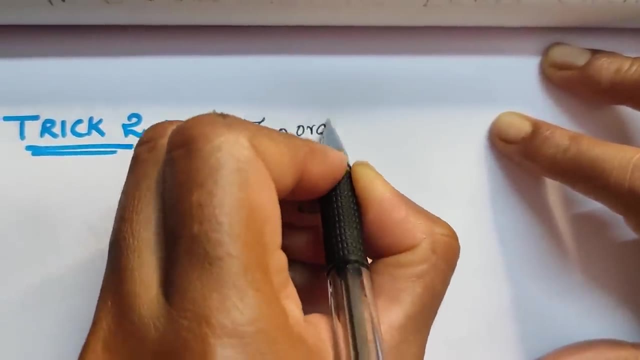 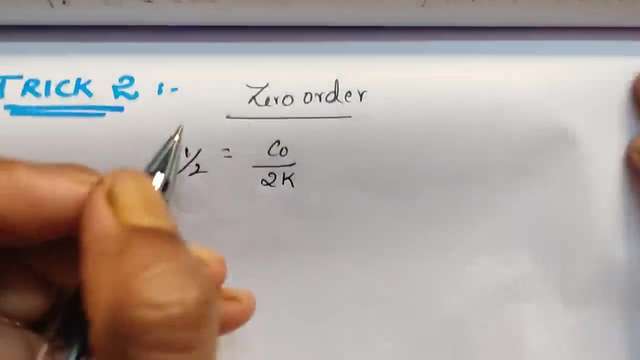 order reaction or for a second order reaction, how to solve those kind of questions I want to discuss with you all here. for a second order reaction, let's say if, let's say if T half is equal to 0, I'm going to write this: 0 order reaction: 0 order T half formula is C naught by 2k. 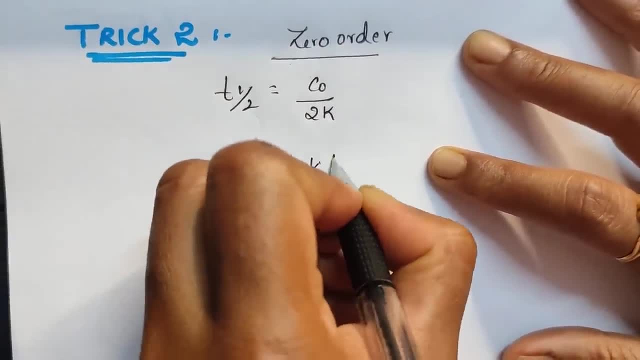 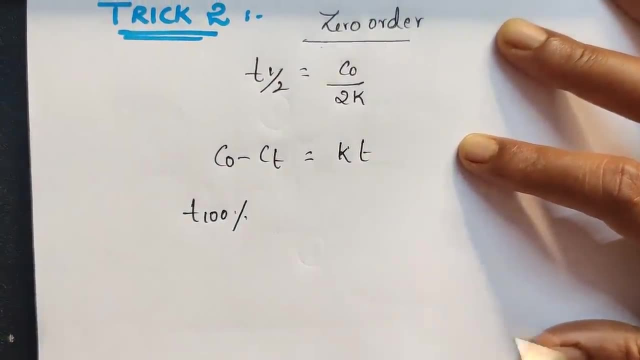 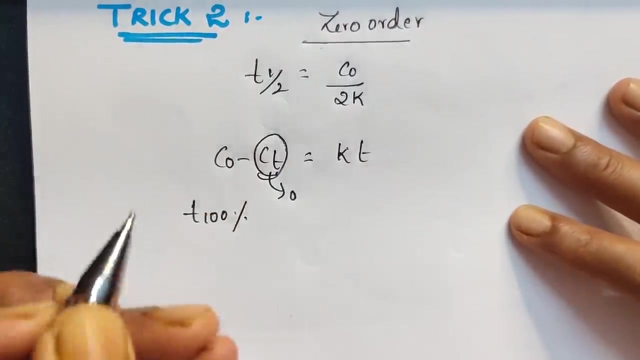 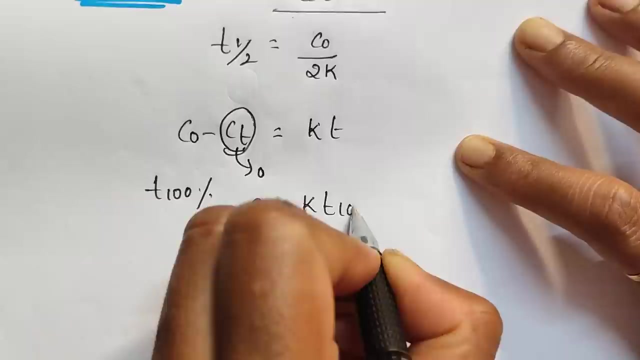 if it is an actually formula, is C naught minus CT is equal to KT. is the formula, if suppose the hundred percent, let us stick: hundred percent it is completed. if 100% it is completed, there will be no concentration of reactants left. keep zero is 100% completed, there is no reactance. then C0 is equal to K. T is 100%, then T 100% is equal to. 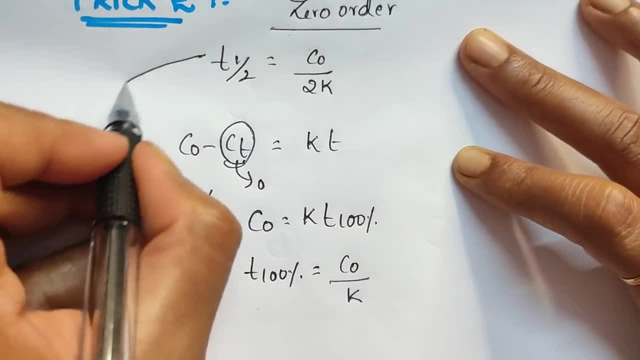 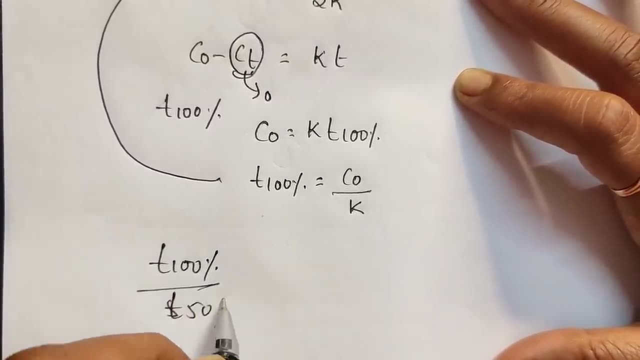 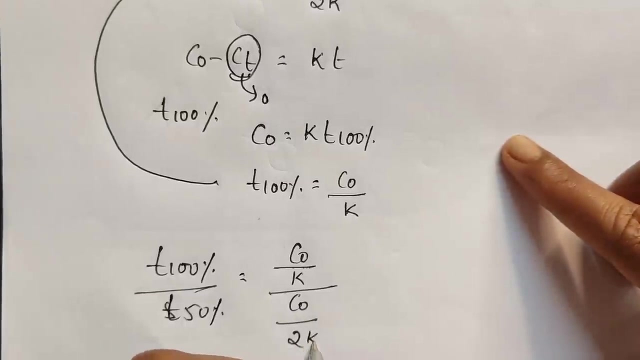 C0 by K. now you want the relation, for example, between these two: T 100% divided by T 50% or T half, which is equal to take these two and divide. this is C0 by K, this is C0 by 2K, then C0 by K. 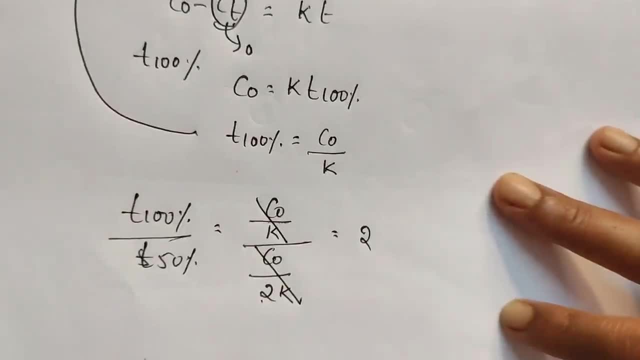 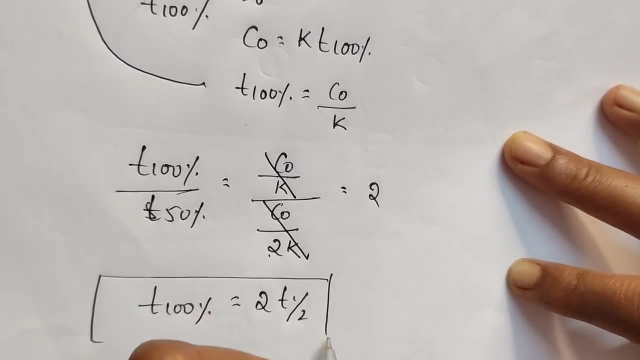 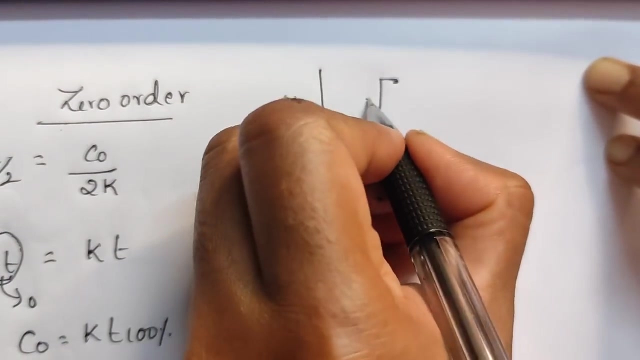 C0 by K. cancel this two comes up, then it will be T. 100% is equal to 2T. half is a formula, right? this is a formula like this. any relation you can find it out. for example, you want for a first order expression. so what is a? what is a first order expression? students? first order rate. 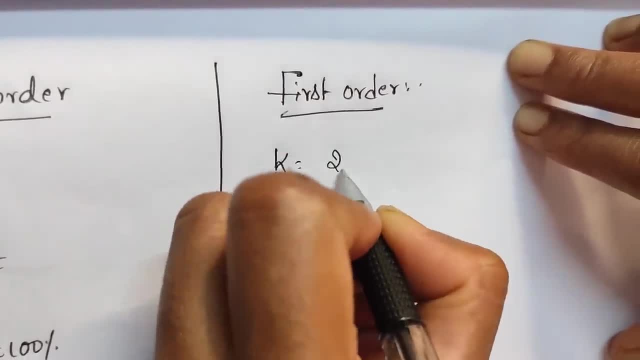 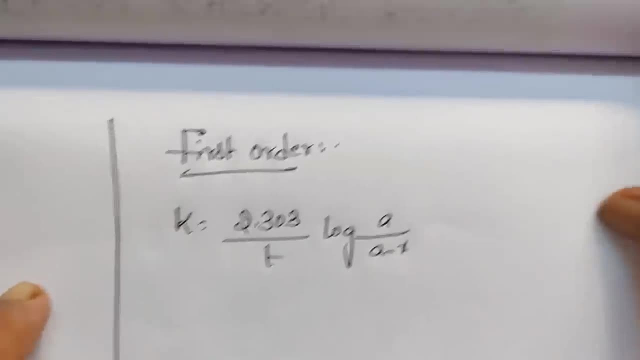 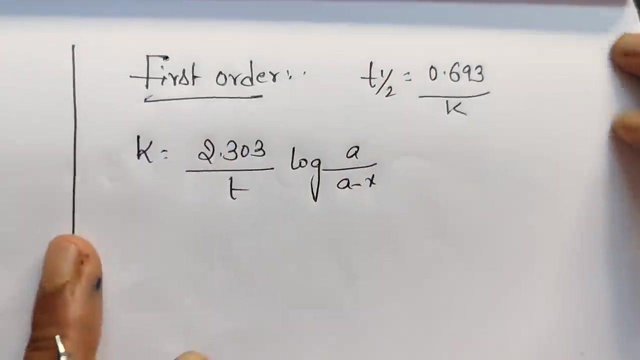 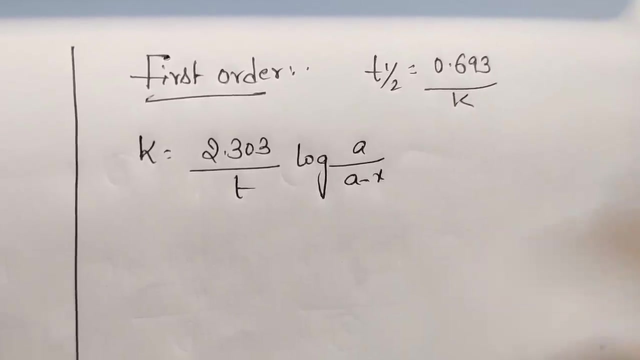 constant expression K is equal to 2.303 by T log of A by A minus X. this is a formula. if you T half formula is 0.693 by K, we get this formula. for example, you want to calculate for 75% or T, 99%, anything whatever you want to calculate, for example you: 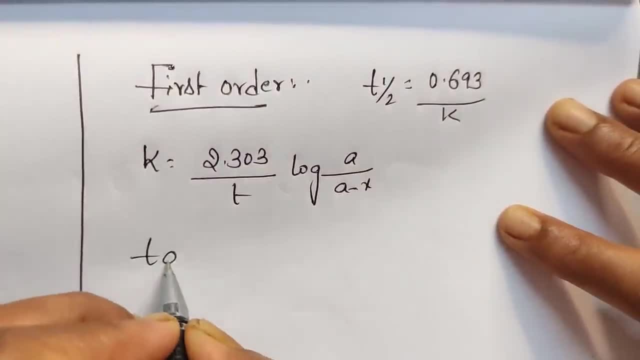 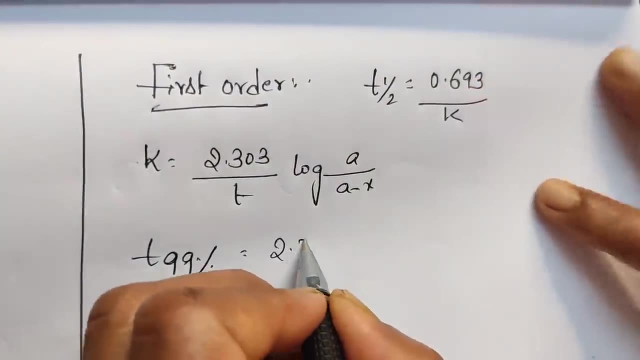 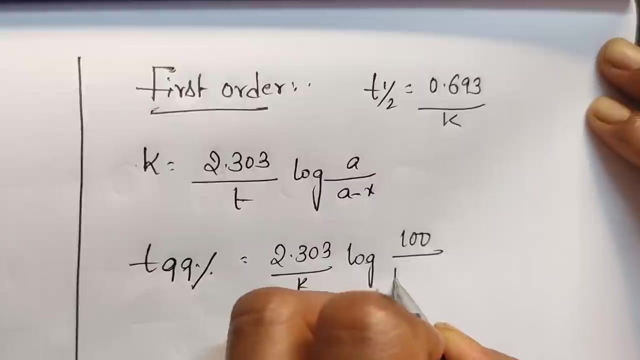 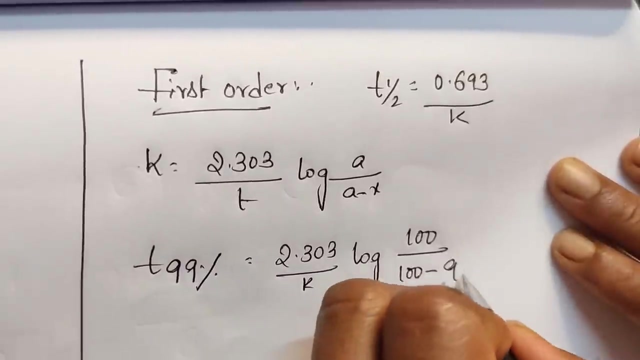 want to calculate T 90 time 99% consumer, then what you have to do is just move this side, K by K. log of initial concentration is hundred divided by 100 minus. if it is T half means substitute 50. it is T 99, substitute 99 e. if it is T 80 substituted: how much ever given in a question? 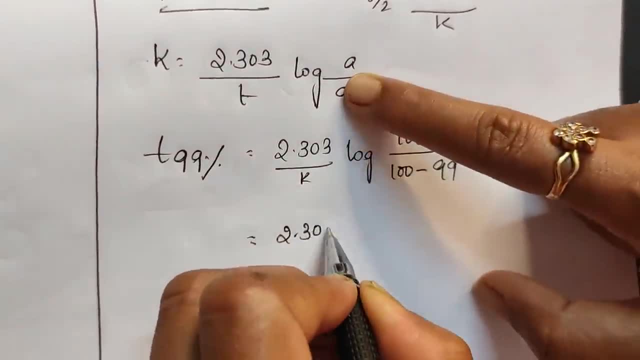 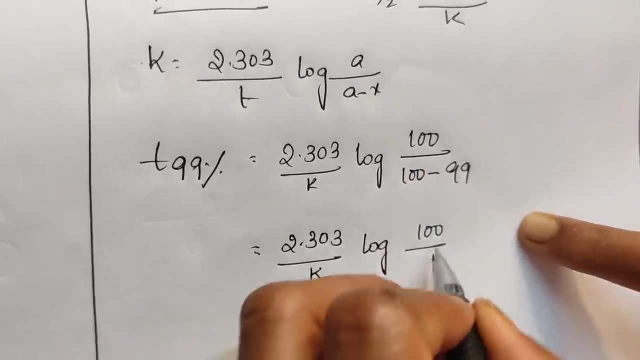 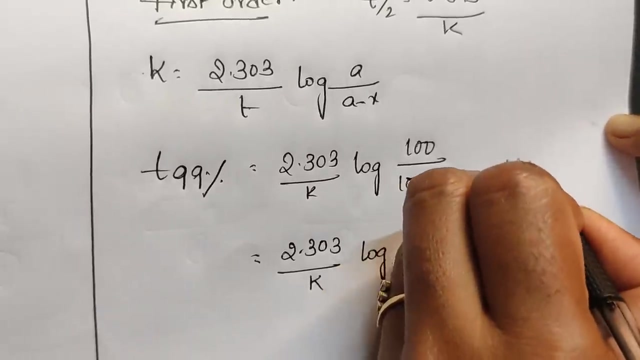 substitute that you know, here only XA place. you substitute that K log. you know, 100 by 100 minus 91, then it is T, up to Cyntathus, even you…. it is 100 means 10, power of 2, log A power B is log A, power B is B log A, then it will. 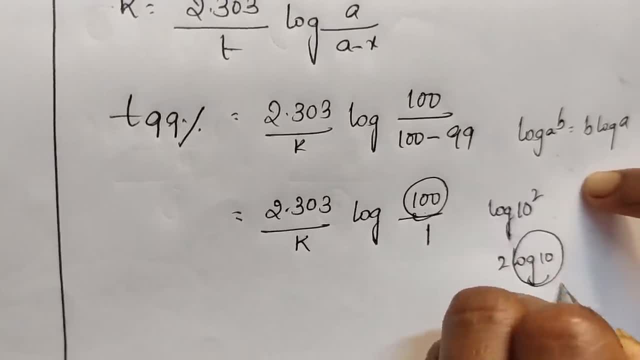 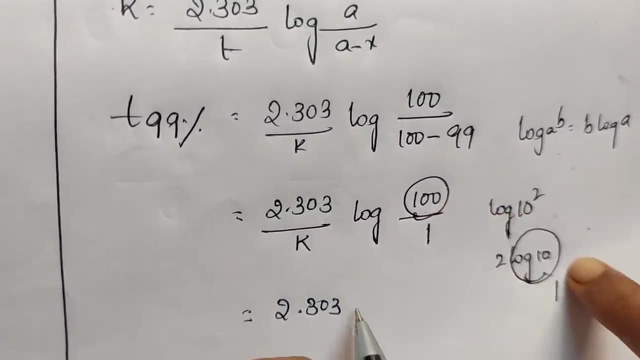 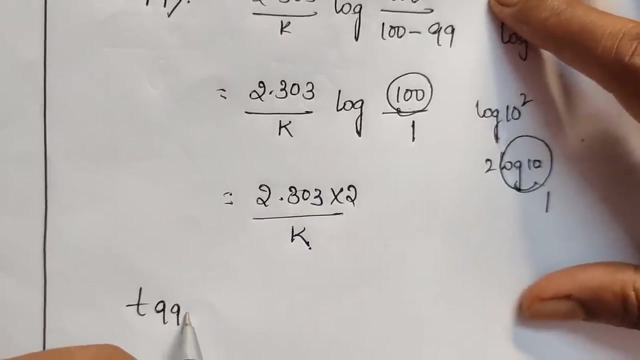 be 2 log 10, log 10 value is 1, so we will be getting here 100 log 2, 2.303 log 100 means 2 log 10, I am substituting here. then, if you multiply this T 99% by T half, which is: 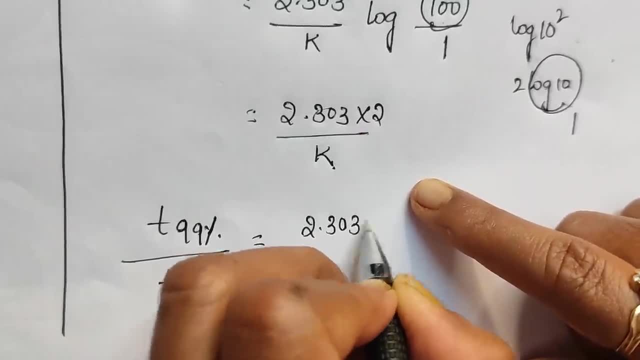 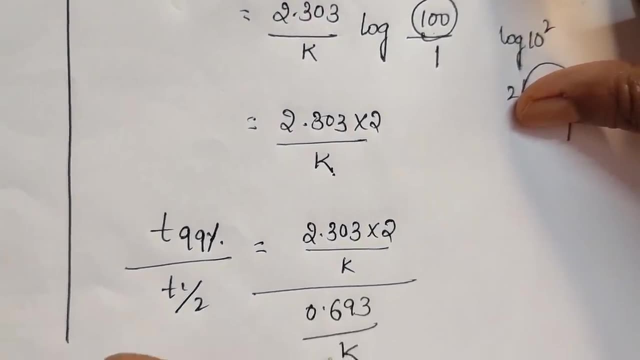 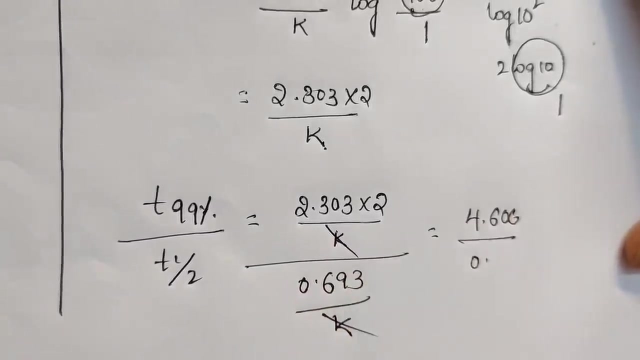 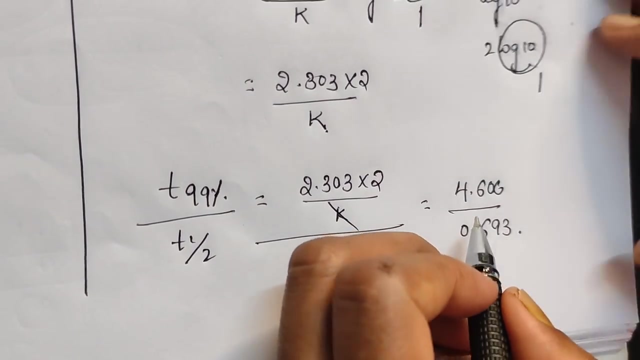 equal. to take this value, 2.303 into 2 by K, divided by 0.693 by K, just to cancel out K, K will be cancelled then 4.606 by 0.693.. So solve this around 6. you will be getting. this is the relation I have taken on my own. 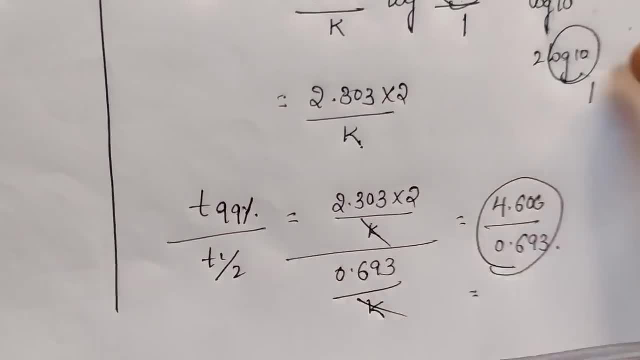 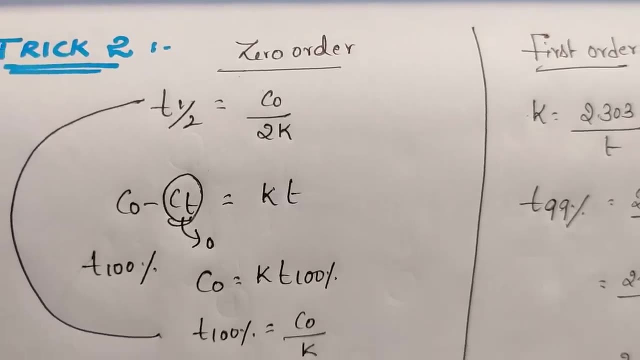 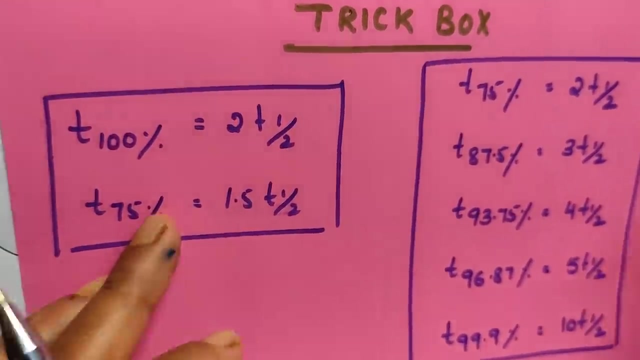 99% any value. you can take it out, but always doing and substituting it takes your time. so I am going to show you the trick box. this is the trick box. whatever the procedure I have shown, you can do like that, but having a grip over all this. formulas: T: 100 power. 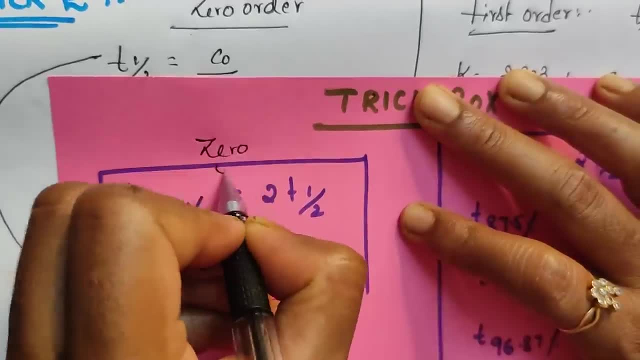 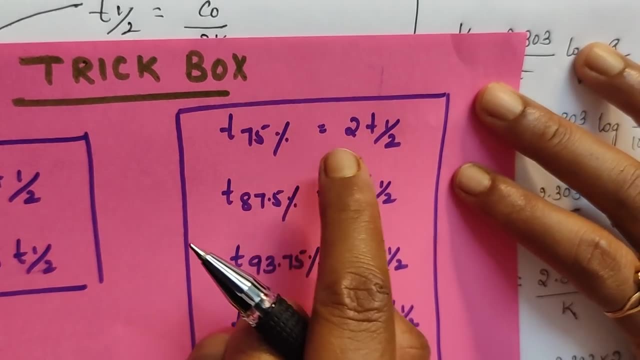 B is equal to 2 T half. this is for 0 order and for 75%. if they ask just 1.5 T half. if you know 75%, they asked this is for a first order, first order. note it down, this trick. 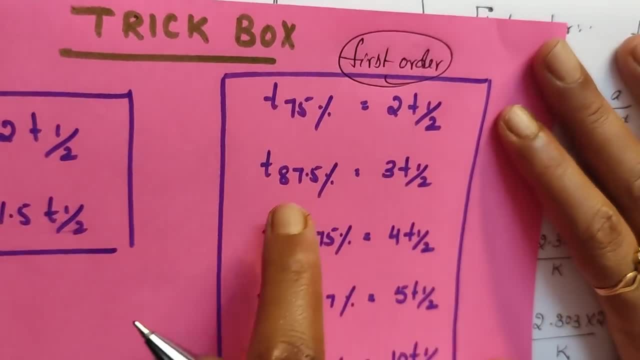 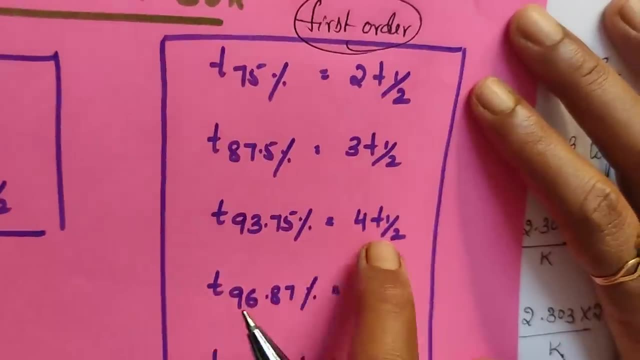 box in your notes. T 75% is equal to 2 T half. 87.5 is equal to 3 T half time. at 93.75% is 4 T half. then this 5 T half, 10 T half. 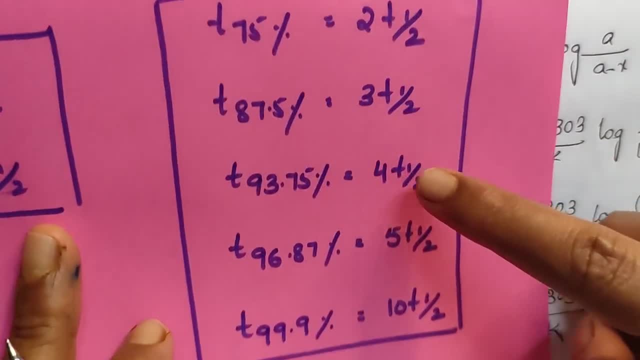 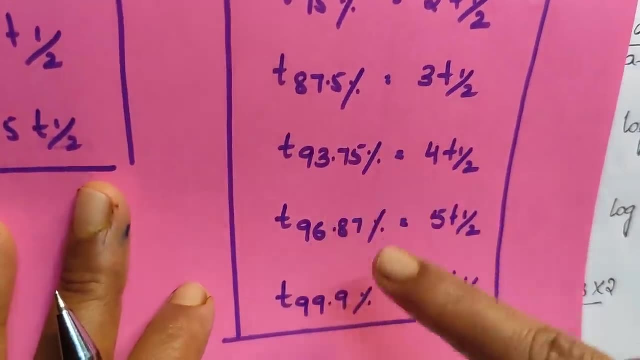 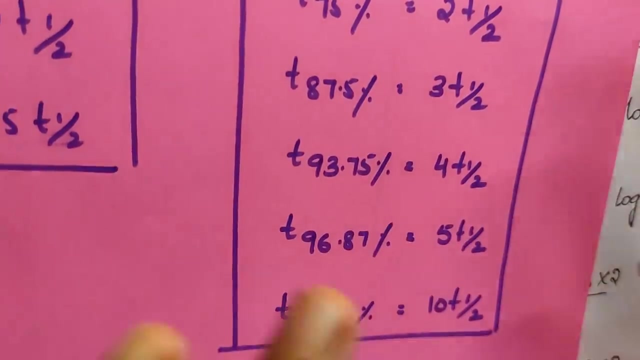 You know, make a note of this, and just you know: 2,, 3,, 4,, 5,, 10,. 2, 3,, 4, 5,, 10,, 75,, 87,, around 93,, 96,, 99.8,. everything is important. 96.87% is also. you have to learn if you don't. 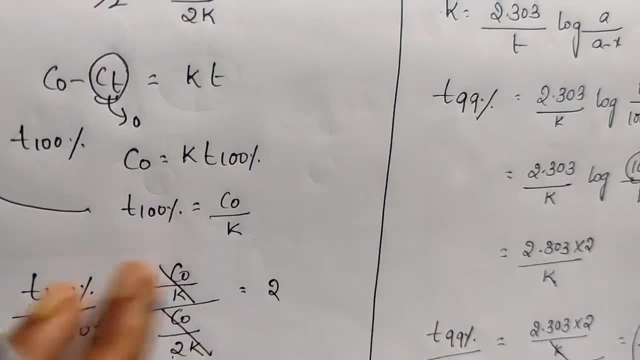 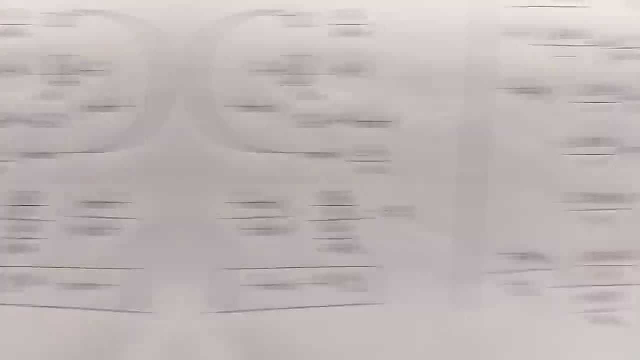 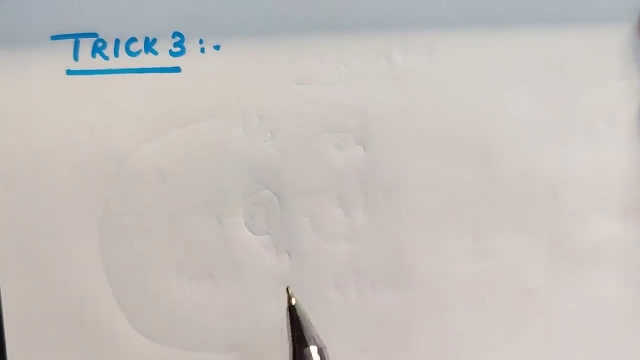 want to learn this trick box, then you need to substitute in this formula and you have to calculate it out. Now let's see trick number 3.. Trick number 3, I want to tell you regarding temperature coefficient. temperature coefficient means if you increase the temperature by either 10 degree Celsius or 10 Kelvin, then rate. 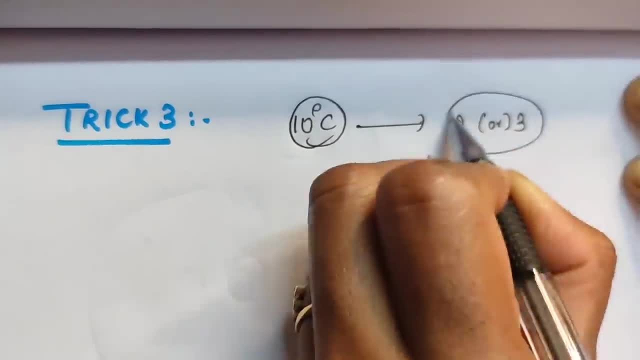 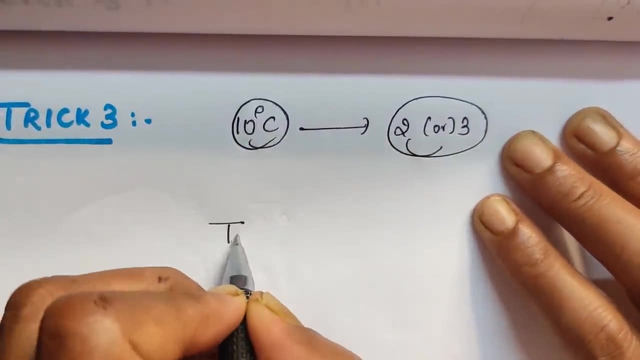 increases either 2 times or 3 times. then they ask the questions based on this. I want to tell you how to solve those type of questions easily by using a simple formula: temperature coefficient to the power of whatever the temperature difference they have given in a question divided. 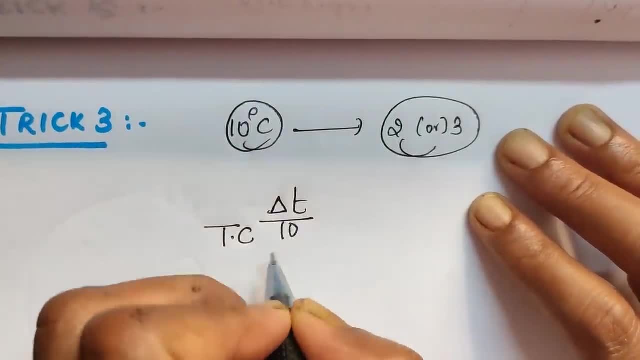 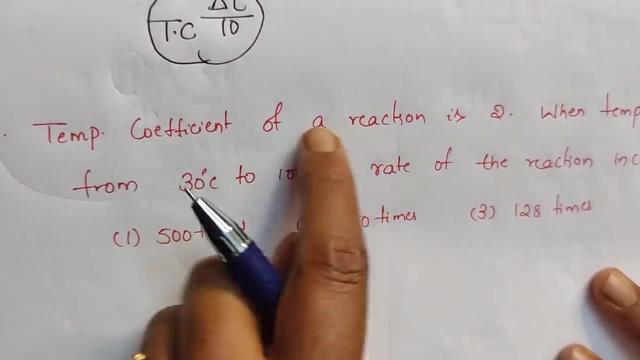 by the temperature coefficient. So the stoichiometric divided by 10 is a formula. Now let us see one question so that you can understand. See the question. temperature coefficient of a reaction is 2 when temperature is increased from 30 to 100 degree Celsius. 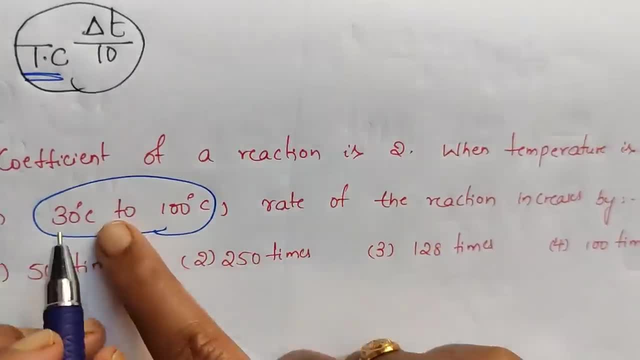 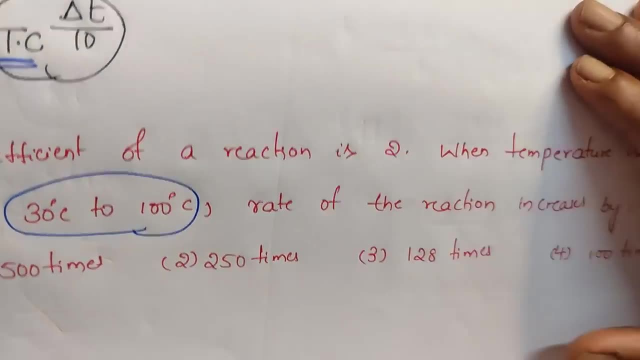 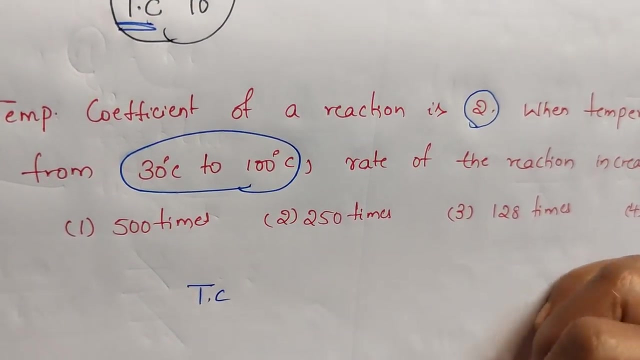 So temperature coefficient value is given 2 and the temperature also. from which range to which range temperature is changing. also, given they are asking, the rate of reaction increases by. So how to do Temperature coefficient? take it here: TEC formula is TEC to the power of delta T by 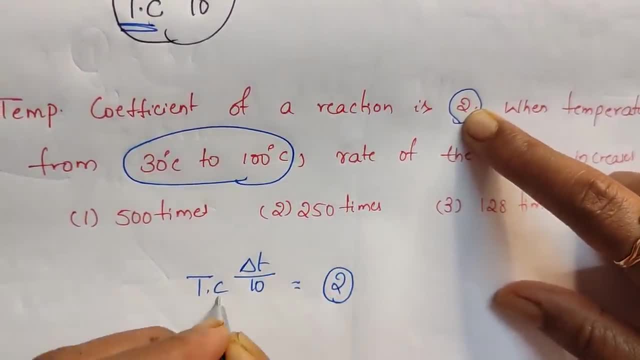 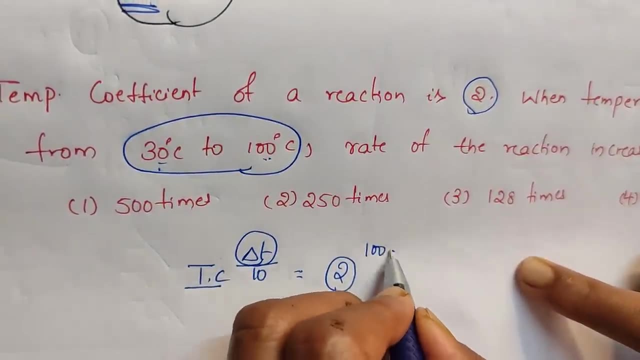 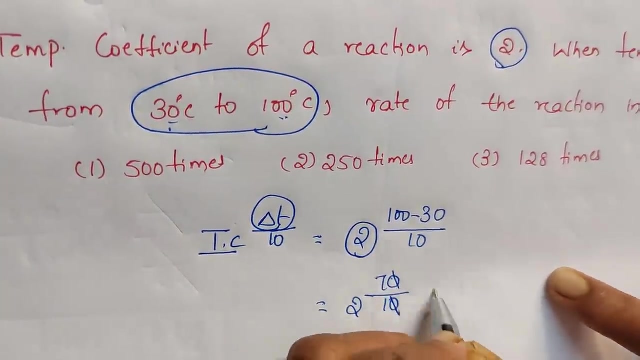 10, temperature coefficient value is 2, take it here. and delta T means temperature difference: final temperature minus initial temperature. 100 minus 30 divided by 10 is a formula. So 2 to the power of 70 by 10, that is 2 to the power of 7, then 2 to the power of 4,. 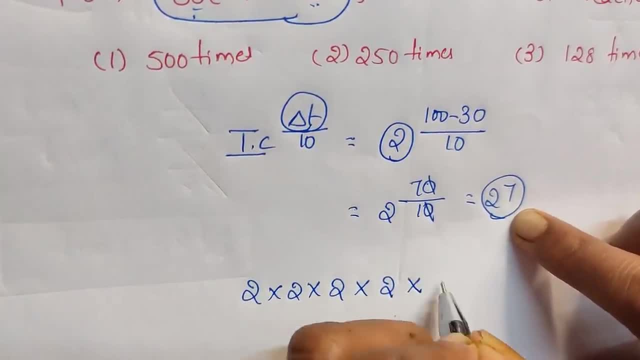 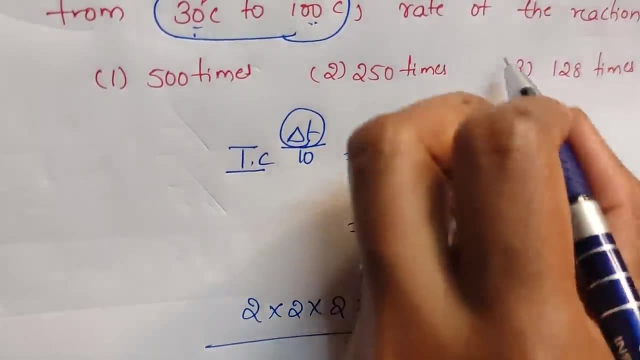 4 to the power of 8.. 8 to the power of 16,, 16 to the power of 32,, 32 to the power of 64,, 64 to the power of 128.. So 128 times is our answer. 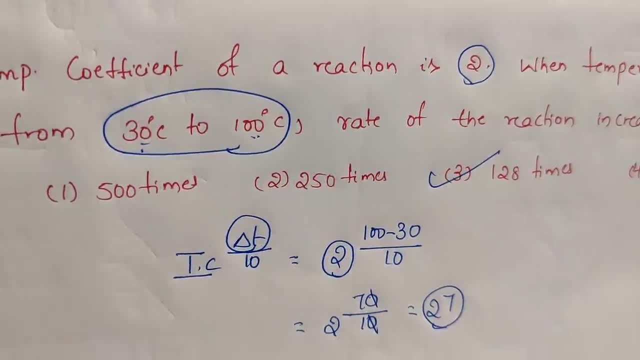 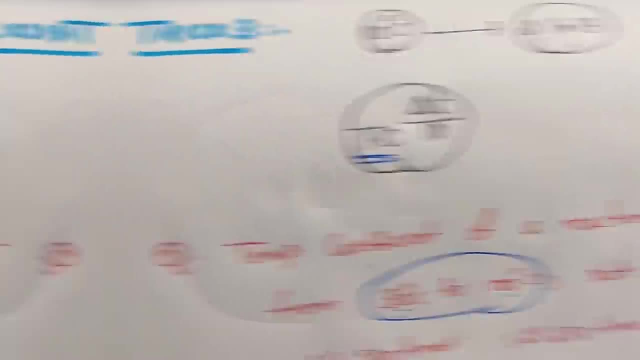 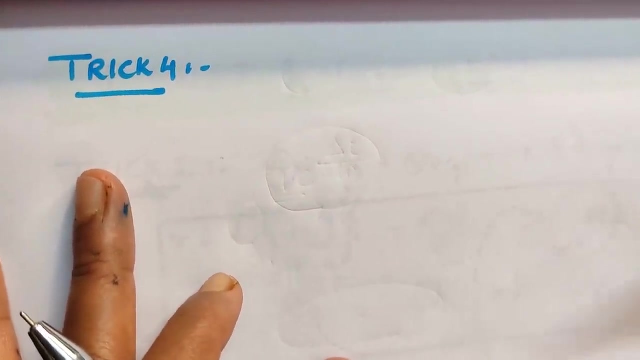 Whatever the difference is given, you need to substitute it. I will give you a test yourself question. Now, before going to the test yourself question, let us see the last trick, trick number 4.. In this I want to discuss with you regarding they gives you initial concentration and a. 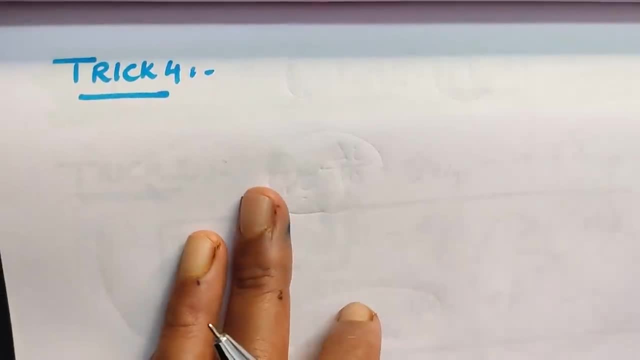 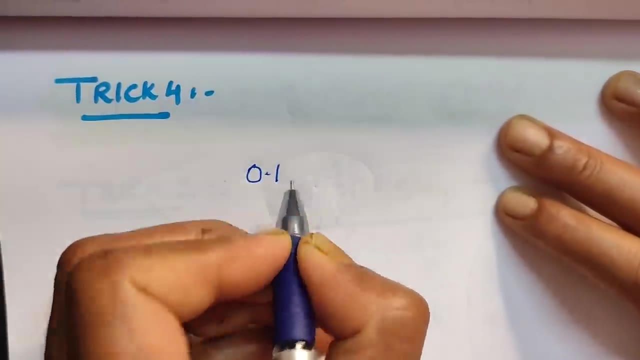 T half. They ask first T half. they give you and they ask you: what is the T half for the next reaction? like you know, initial concentration is 0.1 and then it is changed to 0.05 and then 0.025. 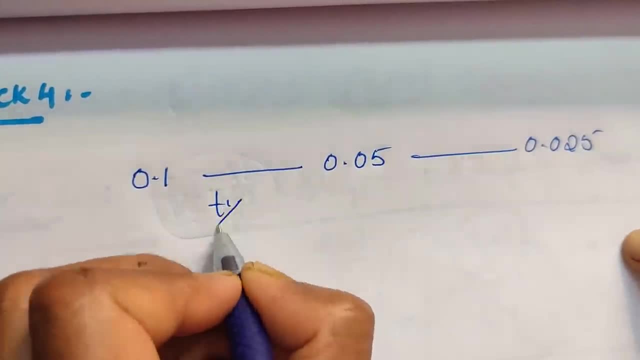 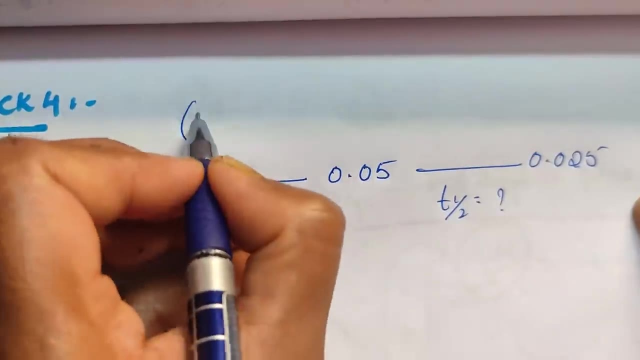 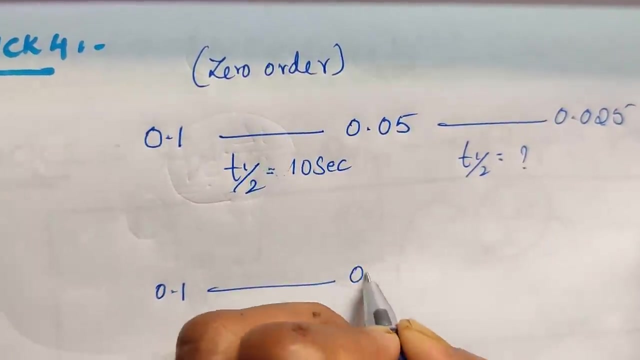 like this and they give you a data like T half here is 10 seconds and they ask you: what is the T half over this, if it is a zero order? reaction, zero order. They mention If it is a zero order or they ask you: it is 0.1, change it to 0.5 and further change to. 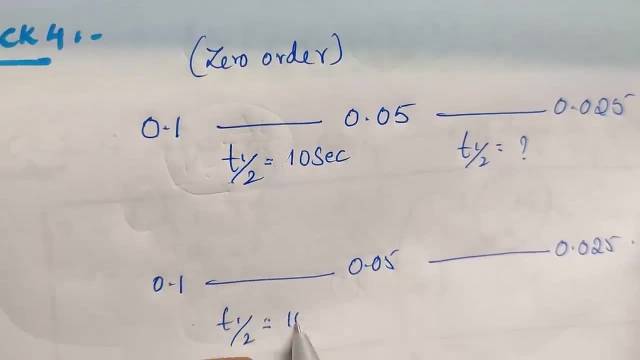 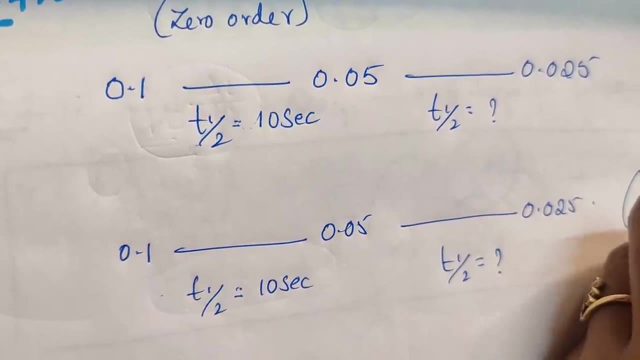 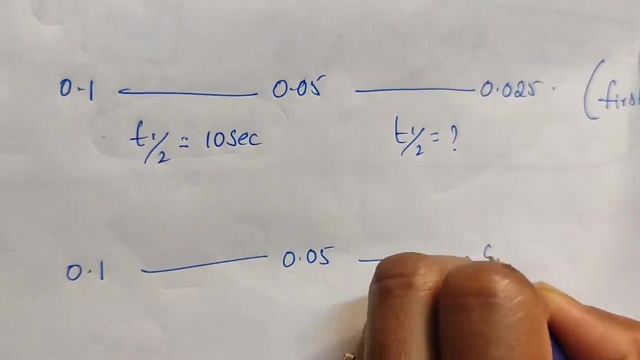 0.25, T half for this reaction is 10 seconds. same question: T half is equal to how much if it is a first order? if it is a first order, or same question, they gives you 0.1 initial, it changes to 0.05 and then to 0.025,. here T half is 10 seconds and then 0.025,. 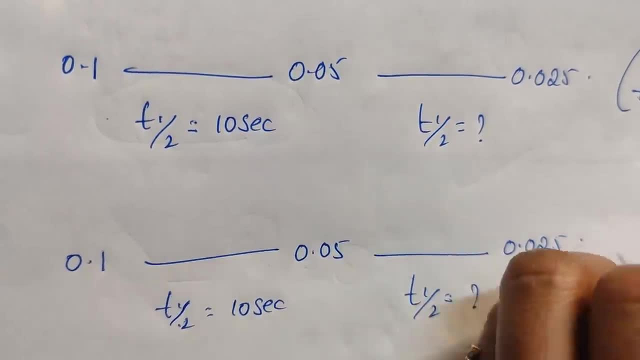 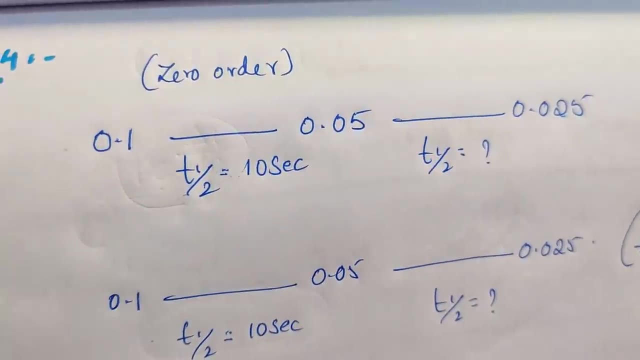 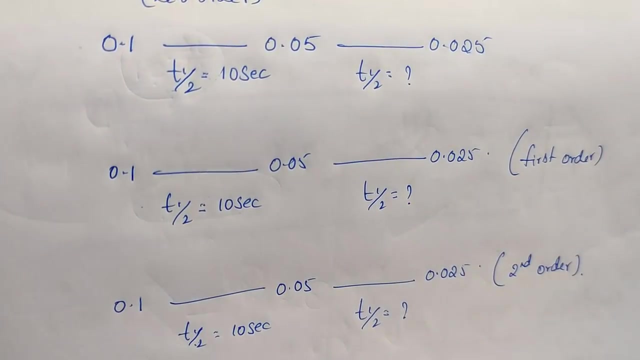 and then calculate T. half same question I am writing here if it is a second order reaction. This is your question: how to solve these kind of questions without using any formula or, you know, without using any formula or any, without any difficulty, in an easy way we can. 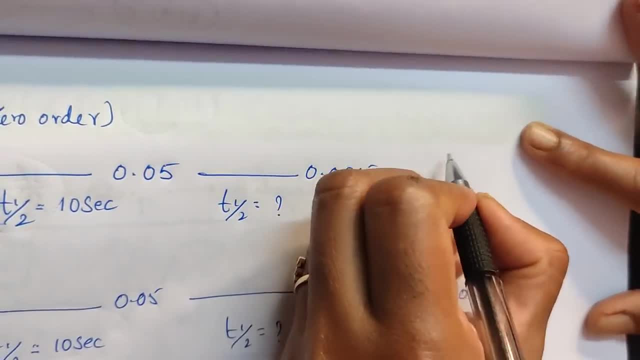 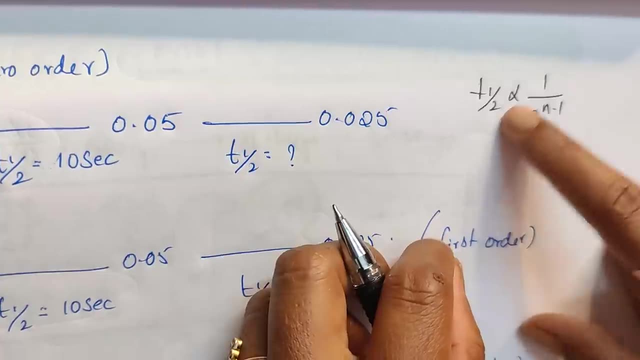 do this one. I will tell you how by using a simple, you know expression- T half, you know- by using the simple formula, you can do it. T half is proportional to 1.5.. T half is proportional to 1 by a, to the power of n minus 1.. 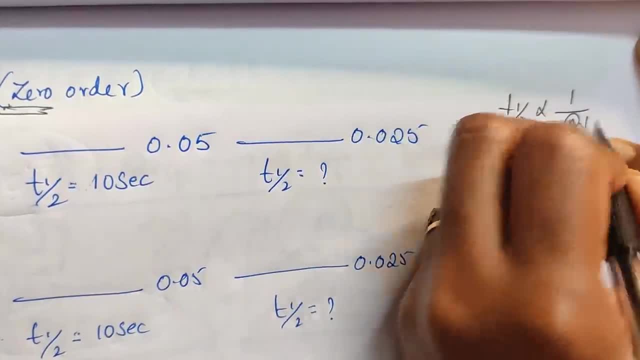 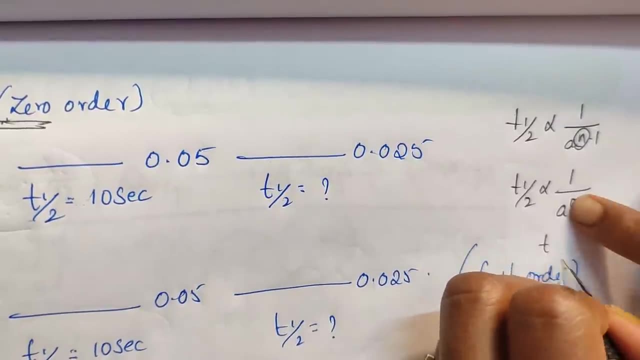 If it is a zero order, C students directly substitute n plus 0. then T half is proportional to 1 by a to the power of 0 minus 1. then here 0 minus 1 is minus 1 if it goes to the numerator a to the power of 1.. 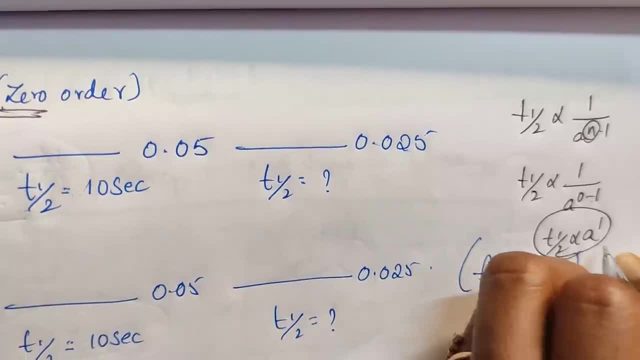 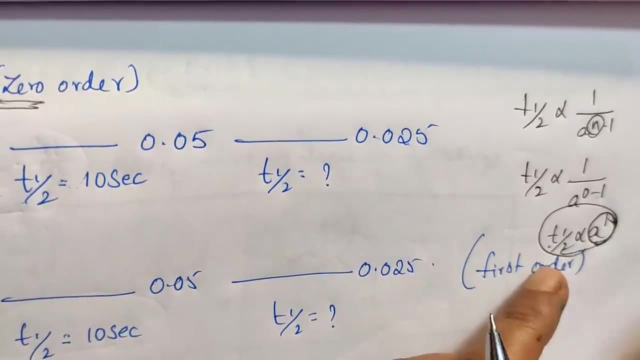 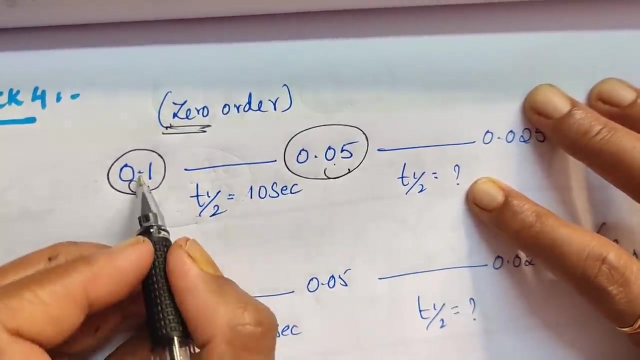 This is the expression we get for a zero order, which means that initial concentration is directly proportional to half life. If initial concentration becomes half, Half life also becomes half. You see, here it is 0.1, it is changed to half. so initial, here initial concentration is 0.1. 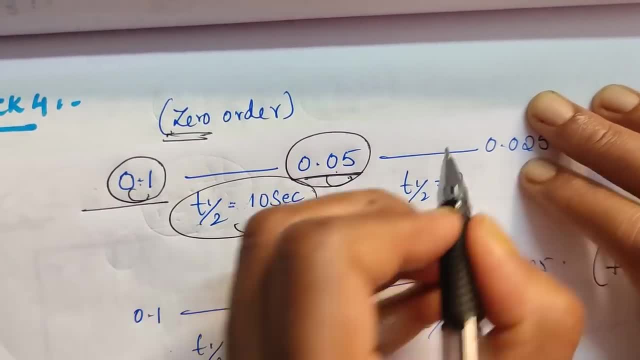 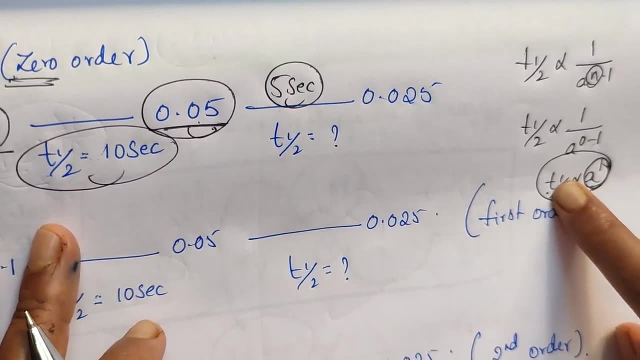 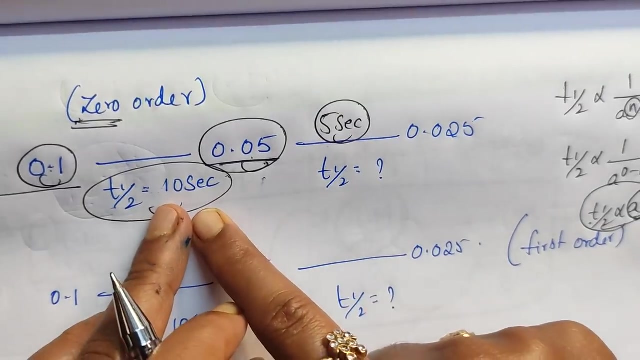 but here initial concentration is becoming half, then T half also becomes half. See again I am repeating: if initial concentration is directly proportional to the half life, here initial concentration is 0.1 and finally 0.05. that time half life is 10 seconds. if initial. 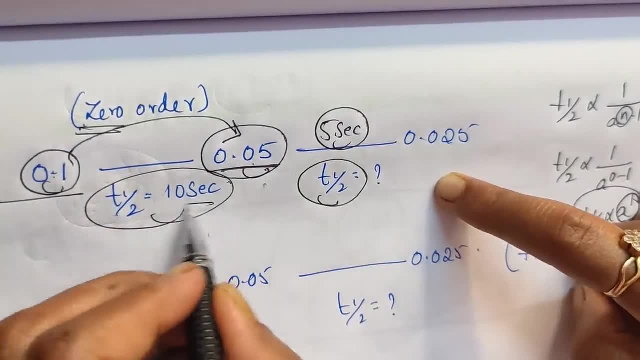 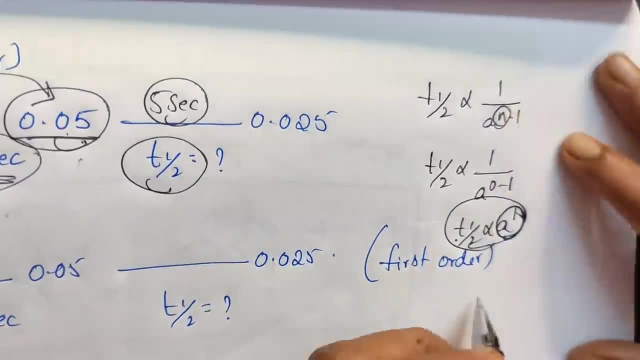 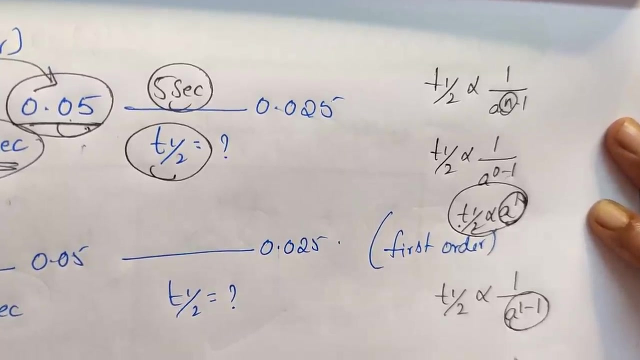 concentration. If initial concentration is becoming half, then half life also becomes half. fine, and now what I do is I substitute for a first order. for a first order: n value is 1, then T half is proportional to 1 by a to the power of 1 minus 1, then it becomes a to the power of 0, anything. 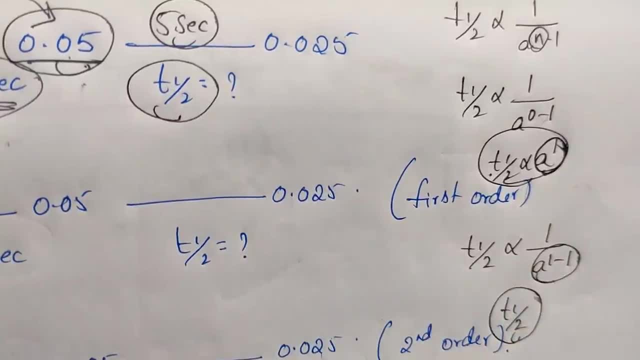 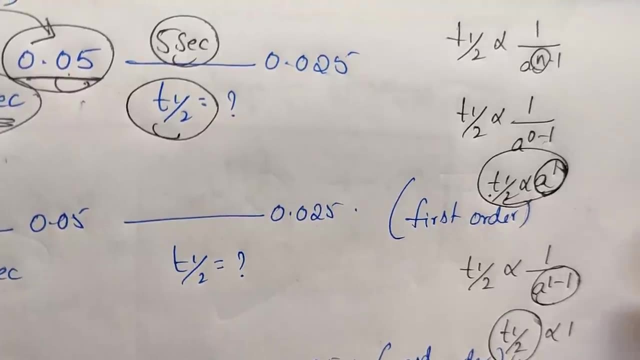 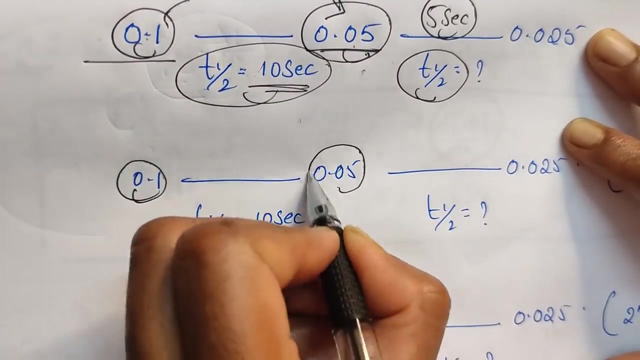 to the power of 0 is independent. T half does not depends on initial concentration, because anything to the power of 0 is 1, so T half is proportional to 1. some constant T half is independent of initial concentration. So here 0.1 is changed to 0.05. so initial concentration is becoming half here, but the 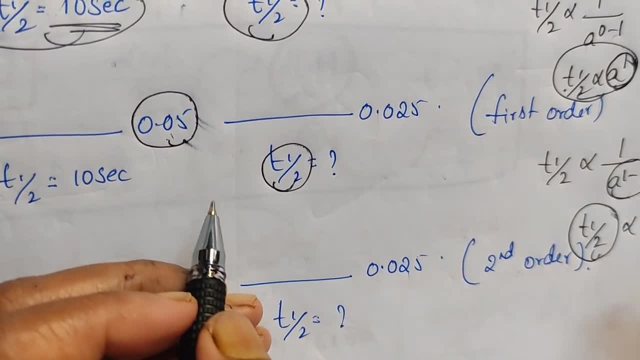 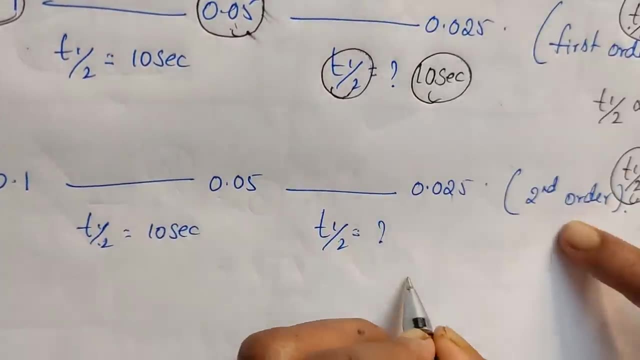 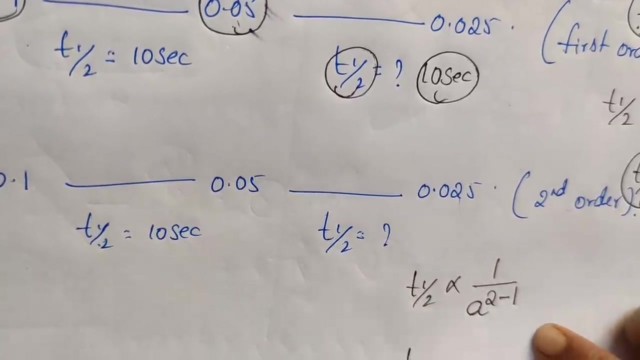 problem is T half does not depends upon initial concentration. so here T half is 10 seconds. and coming to the second order, T half is proportional to 1 by a, to the power of n minus 1, so n place substituted 2.. Then T half is proportional to 1 by a. 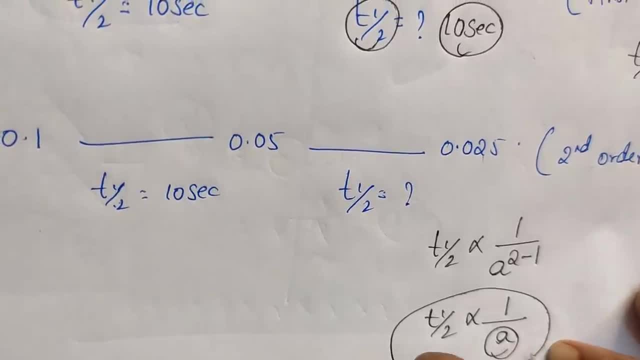 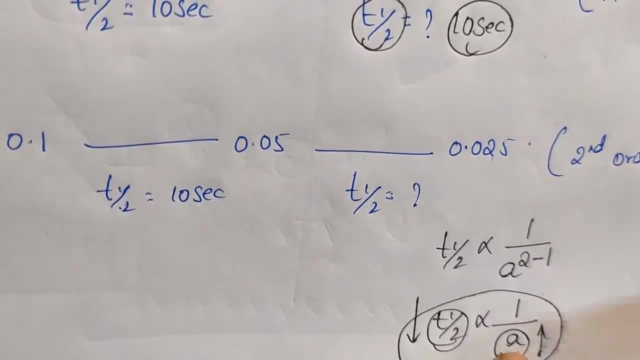 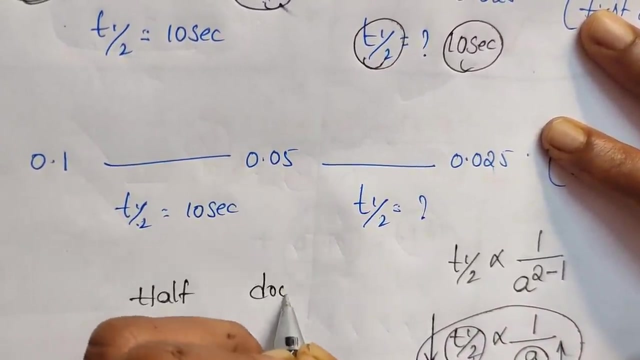 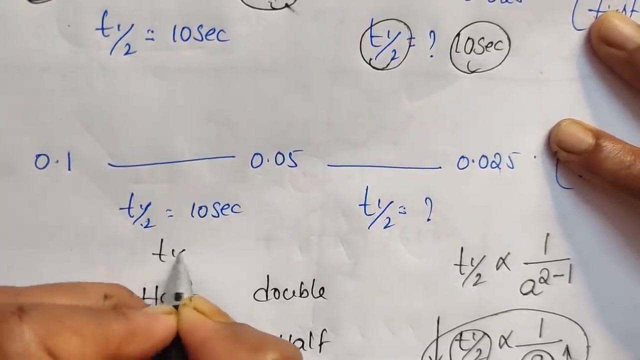 Which means That if you increase a initial concentration, if you double it, half life becomes half. if you increase, if you half the initial concentration, half life becomes double. if you half it, it becomes double. if you double it, it becomes half. this is the formula. this is T, half this. 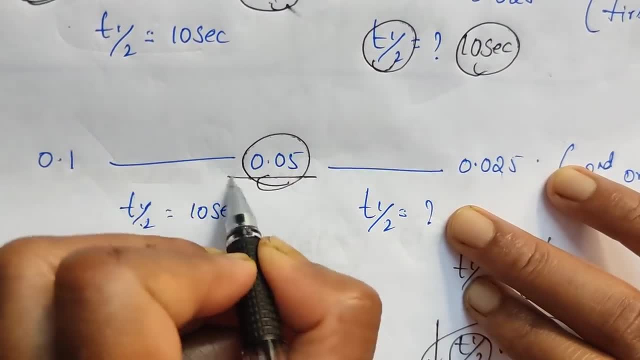 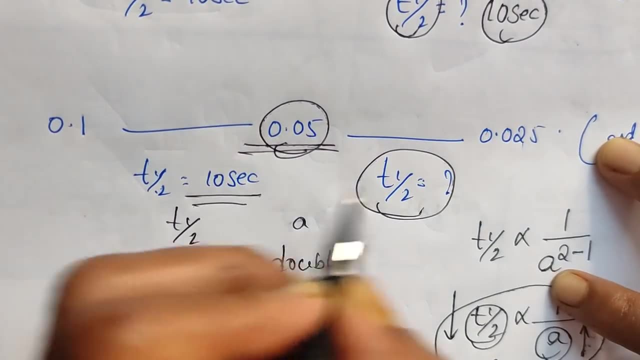 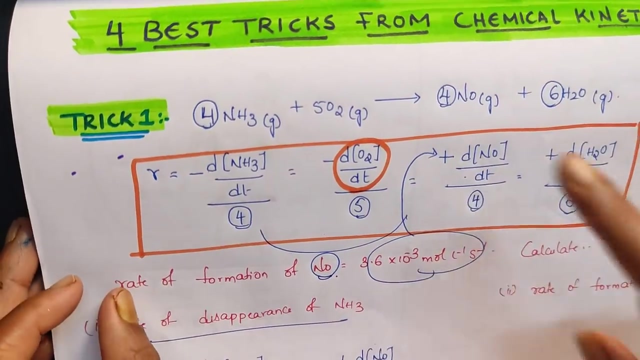 is initial concentration, So initial concentration becomes half. So time period- Initial concentration becomes half, so half life becomes double. so 10 seconds double means 20 seconds. Now let's see the you know? test yourself questions In a trick. number one, I discussed rate expression. regarding a rate expression, how? rate of formation?